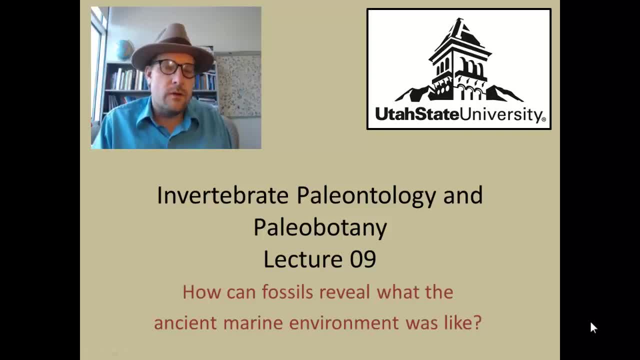 be talking about paleoecology and how we can use the fossil record to reconstruct what the environment was like. In this lecture, we are going to focus on the marine environment Before we go into too much depth with reconstructing the marine environment using fossils. I wanted 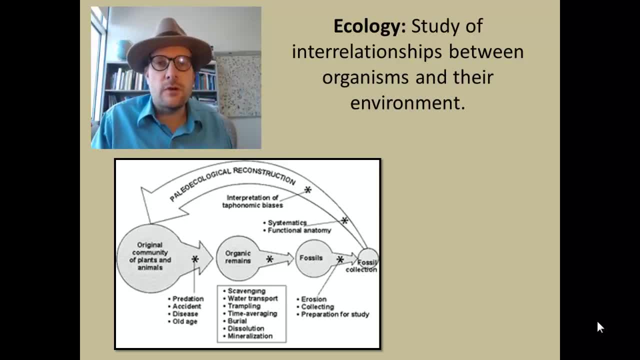 to go through a couple terms, particularly in this lecture, to get us thinking about the marine environment and how animals and plants and organisms exist together in the fossil record and how they do that in the modern record as well, and sort of understand or detangle these complex relationships between various organisms. This is all part of the 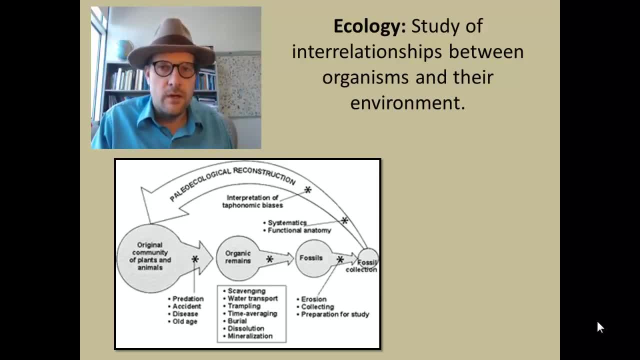 science of ecology. Ecology is the study of interrelationships between organisms and their environment. Understanding what organisms you have present in the fossil record will tell us a little bit about what the environment was like, and so that is the key of doing these types of studies In ecology: you can go out to the actual environment and you can make observations. 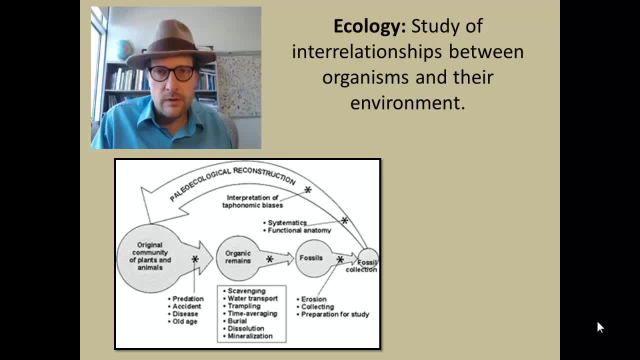 you can collect species, you can analyze whatever you can see in the natural modern environment. With fossils we are basically getting sort of the fractal structure of the environment. There are fragments of fossils that are preserved throughout a series of processes. So in this figure down here we see that we start with the original community of organisms. 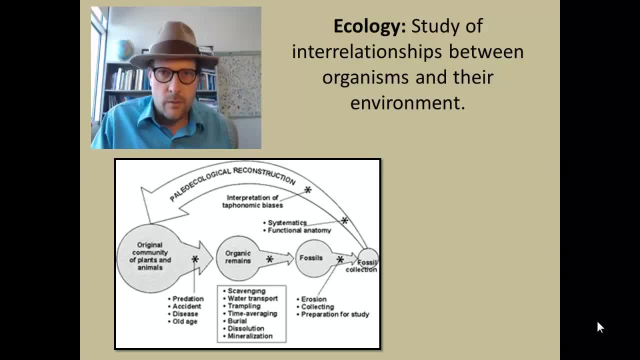 of plants and animals. from that we are dealing with only the ones that have died their organic remains, from that, only those ones that have been fossilized, and of those, only the ones that have actually made it into a fossil collection. Paleoecological reconstructions rely on the 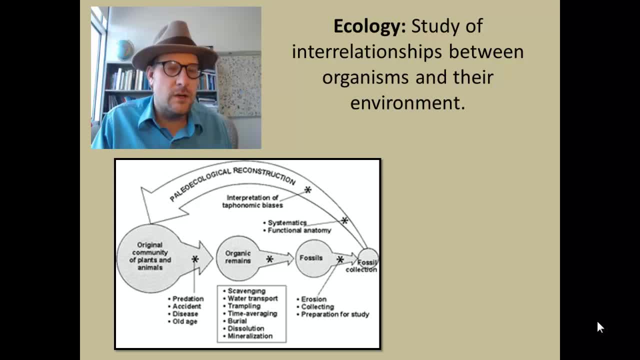 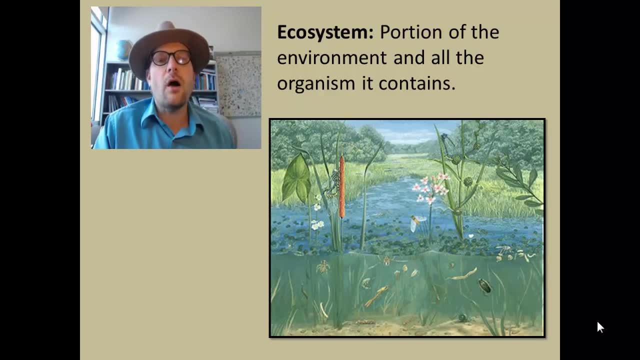 attempt to sample as much of the original community as possible. What you want to do is reconstruct the ecosystem. The ecosystem is a portion of the environment and all of its organisms that it contains. So to recreate the ecosystem of a particular rock unit, we are going to have to try to find as many fossils and diverse fossils that 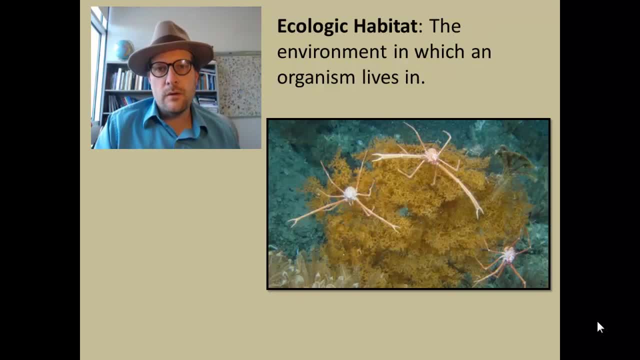 we can find in the rock record. There are a couple of other terms that I want to define. The first is ecological habitat. Habitat is basically the environment in which an organism lives in. This is like the address or house that the organism lives at. It is basically the type of environment that these 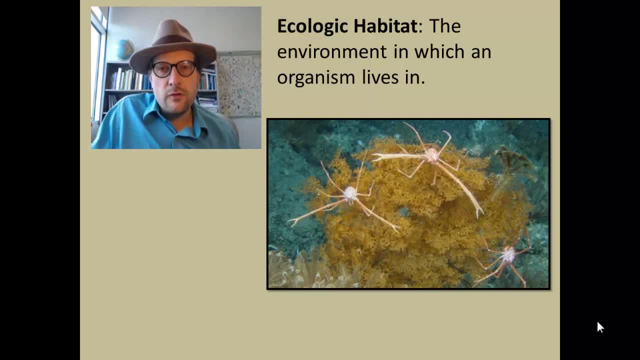 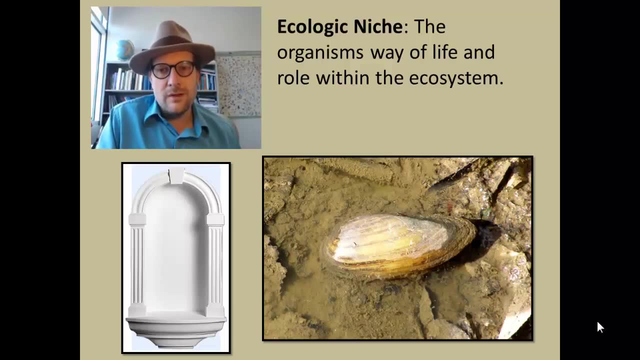 organisms find themselves in Habitat can be contrasted with ecological niche. The niche is basically the way in which the organism fulfills its duties, its way of life or role within the ecosystem. Niche comes from the term for niches like you put into a wall. 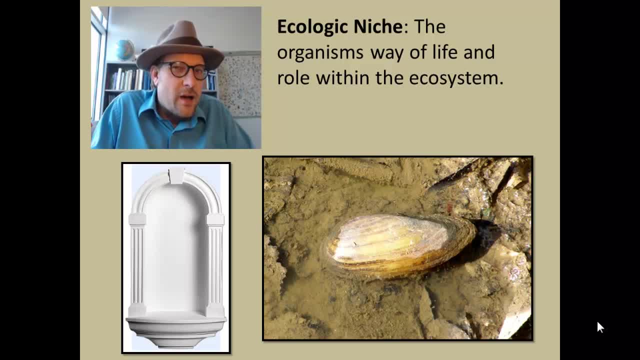 The niches are basically the job or the duties that the organism provides. For example, with these clams, it is a filter feeding organism that filters out various microorganisms within the mud or substrate, Whereas there might be other niches that might be carnivorous. 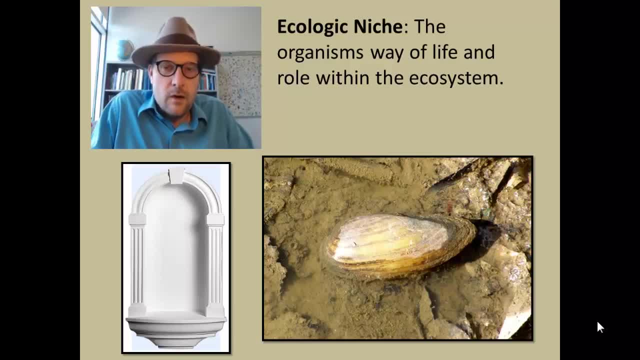 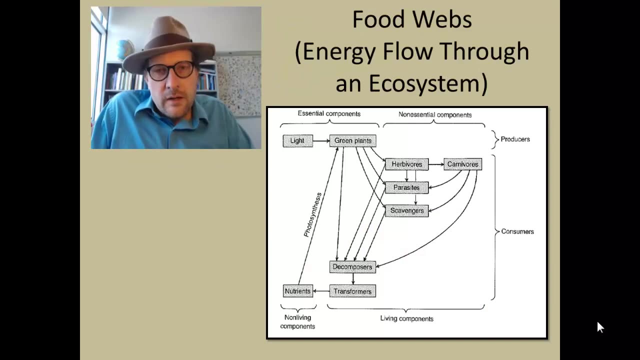 animals, herbivores or grazers. These are all types of ecological niches that are the way in which the organism survives. organism is able to function and survive in the environment. Another thing ecologists are really interested in, and less so in paleoecology, is figuring 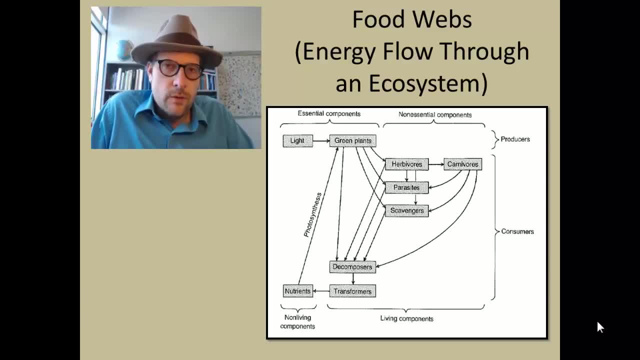 out food webs or the way in which energy flows through an ecosystem. You've probably been introduced to food webs in an introductory biology class or from high school or even junior high, where food webs are basically how the energy, the nutrients in the ecosystem is transported between various organisms. 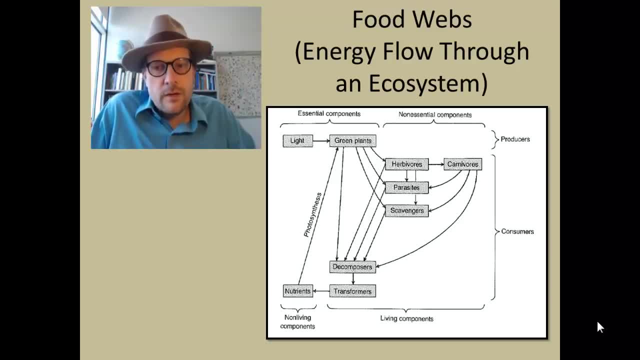 This is where you have herbivores, where they are eaten by carnivores and the carnivores can be scavenged on other things. So it's basically following the energy through a complex series of relationships. Now, food webs are really difficult to reconstruct using the fossil record, in part because often 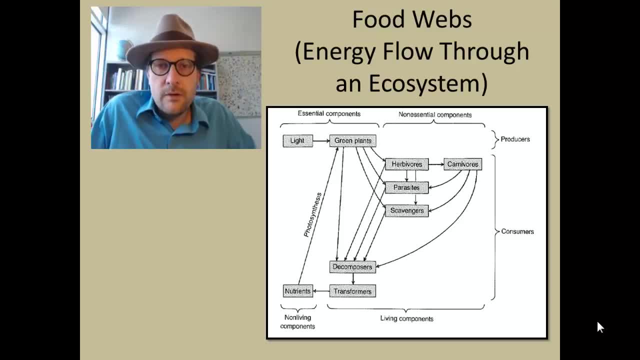 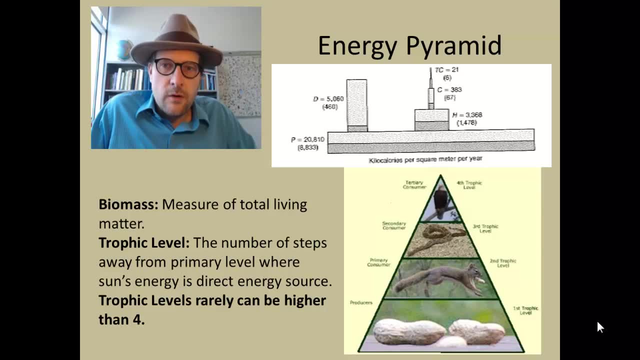 times you're missing some of the key components of food webs, including many of the primary producers, which you may not necessarily see in the fossil record. Also related to food pyramids, There are energy pyramids where we take the total biomass which is measuring the total. 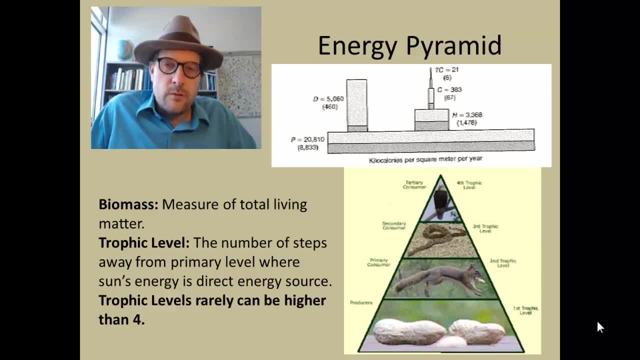 amount of living material and then you categorize how far away they are from the primary producers. The primary producers are those organisms that derive their energy from sunlight or chemical reactions. Primary producers don't necessarily need to rely on other organisms to survive. We have primary producers, primary consumers, secondary consumers, tertiary consumers. 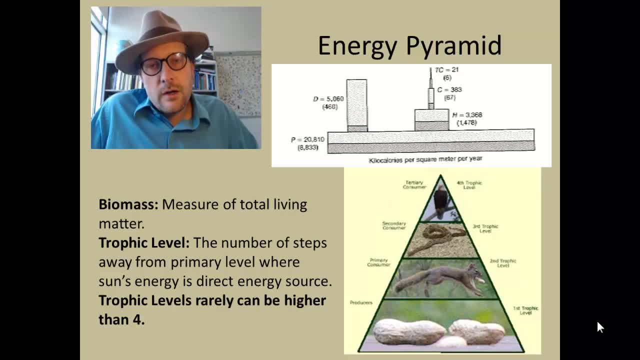 As you move up the energy pyramid, at the tip are going to be organisms which rely on the previous and they oftentimes will quickly narrow down to a very small amount of biomass. Think about this example where we have eagles at the top, snakes, squirrels and peanuts. 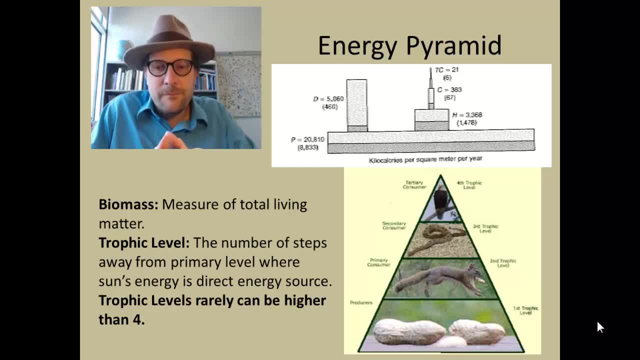 There's going to be a lot more peanuts In terms of biomass compared to squirrels, and there's going to be a lot more squirrels in biomass compared to snakes, and there's going to be a lot more biomass of snakes compared to eagles. 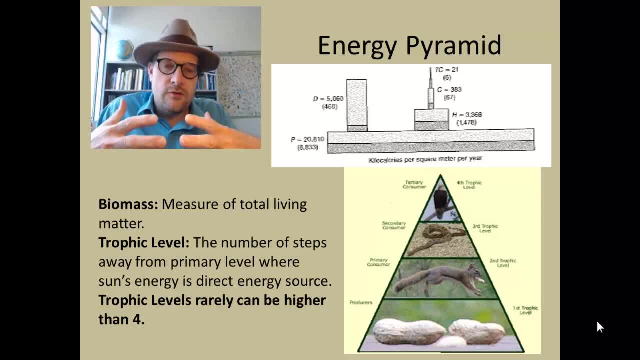 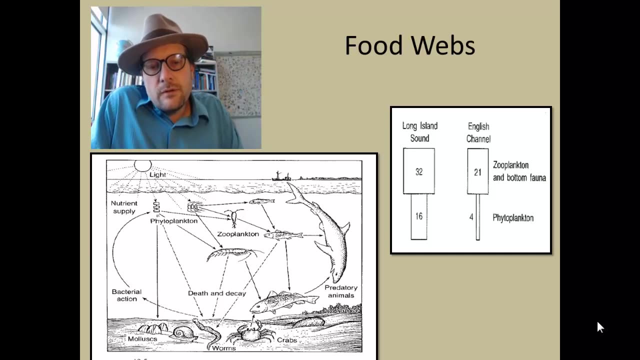 The higher you are in these trophic levels in the energy pyramid, the smaller the amount of biomass. Trophic pyramids are usually not very high. Once you get about four or five, you really just don't have enough energy. Reconstructing food webs can also help you. 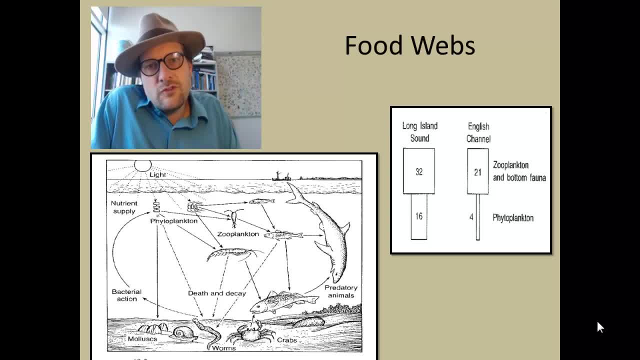 A little bit in the terms of understanding how much energy is entering into the system. This might be something interested in paleontology, when we're comparing geographic places or trying to reconstruct what the climate or the environment was like. Here's a comparison of the diversity of various organisms in a food web where we can classify. 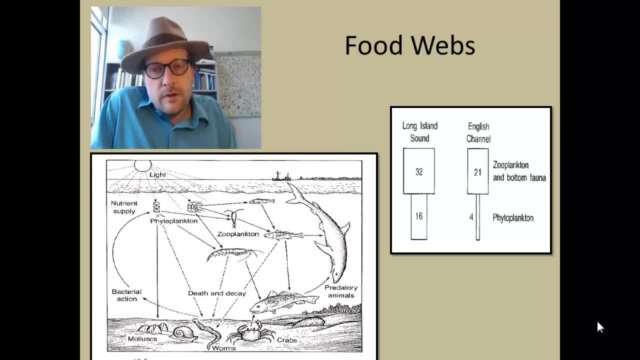 phytoplankton and zooplankton. In a final study we're looking at the English Channel and Long Island Sound and you can see there's greater diversity within the Long Island Sound than there is in the English Channel, indicating that there is probably more energy or more light hitting the Long 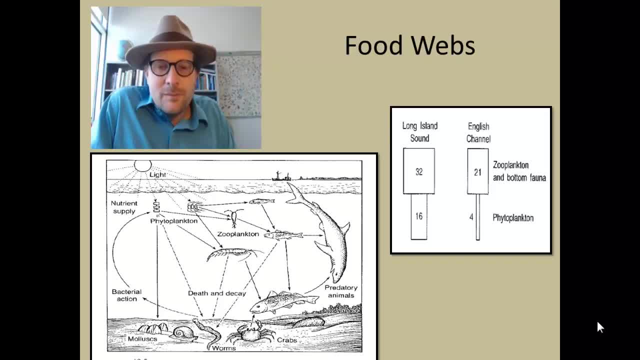 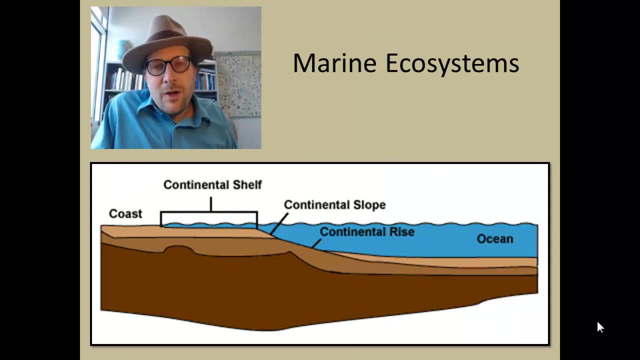 Island than the English Channel, which tends to be a little bit cooler. Understanding these sorts of food webs will give us a better insight of what the environment was like and we can reconstruct this based on a fossil record and looking at these comparisons and reconstructing the food webs. 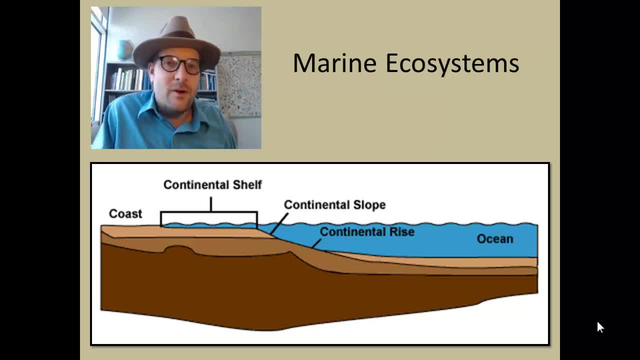 We live on land, So many of us are probably not very familiar with what the marine ecosystem is. In the next few slides I'll talk a little bit about the different terminology that we use for the different parts of the marine ecosystem. This is a very simple diagram showing the transition from a coastline into the open. 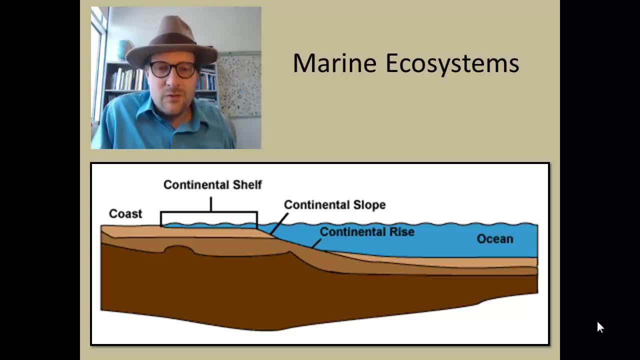 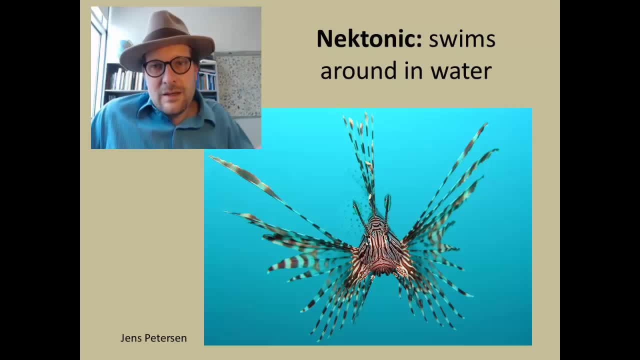 We can divide up this transitional zone into the coastal zone, which is a shallow ocean that sits on top of the continent. We can divide up this transitional zone into the coastal zone, which is a shallow ocean that sits on top of the continent, that really swims or actively swims in the water column. we refer to this as nektonic, like tonic, are organisms that float around in the water. they may have very limited ways in which they can basically swim around. so this is an example of a jellyfish where they are first floating kind of free floating in the water column. they have very limited control on the direction that they're. 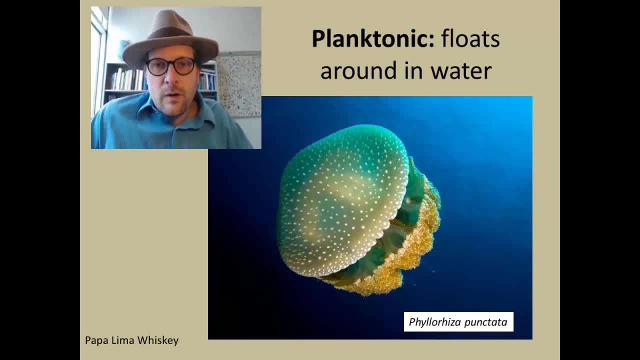 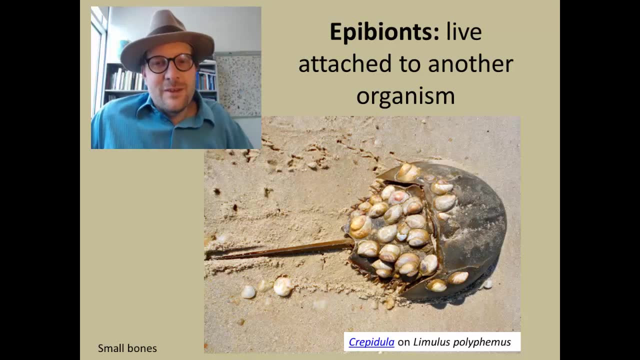 moving around. they're just floating in and existing in the water column we call the planktonic condition. so they're just floaters. epibots are probably the coolest things. these are organisms that lived attached to other organisms, and we'll be talking a lot about epibots later on. so these are some examples of 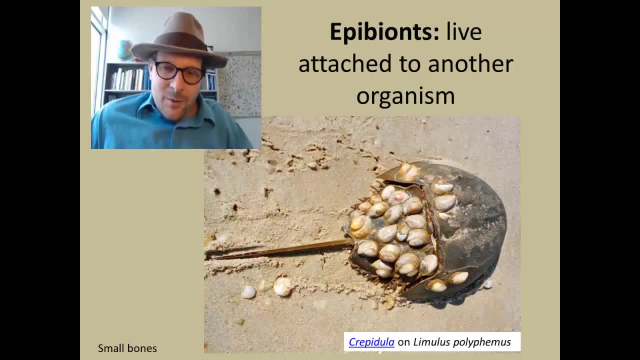 some shells of crept, Ella on a horseshoe crab, and so there's a lot of organisms that will live on other organisms, and we'll be exploring a lot of organisms that make the living by just hitching a ride with some other organism and that 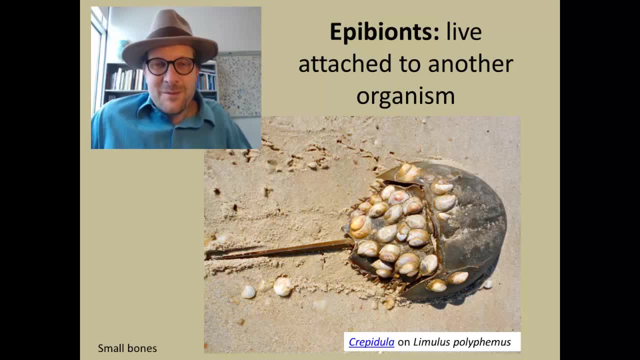 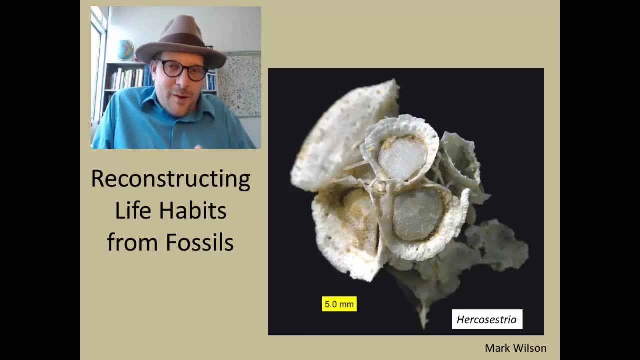 way they can be sessile, but they can also move around as well, as little talk about later on. so there's lots of really good organisms, of epibots. so I want to talk a little bit about sort of amazing fossils where we can sort of reconstruct their 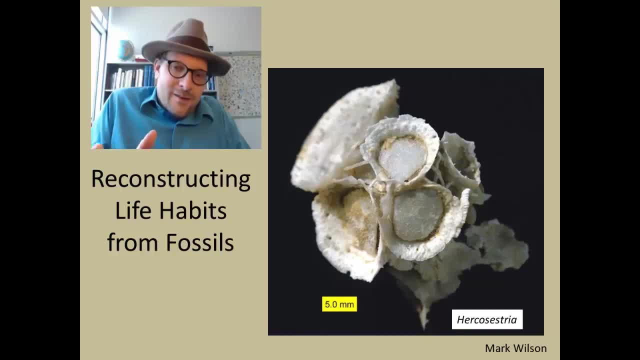 life habits as a fossil and in this give us some greater insight in how they're making their living, and then later on in the next video in lecture 10, talked a little bit more about how we can use the fossil record to look at perturbations in 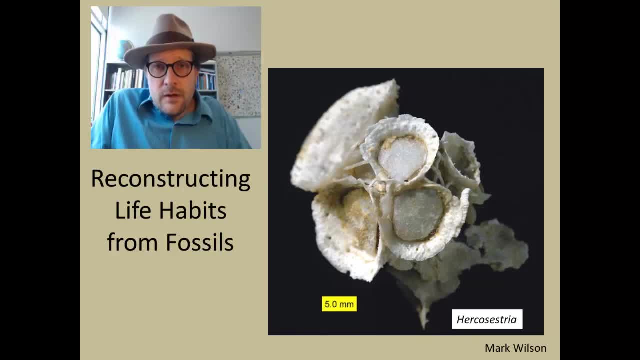 the fossil record and recovery intervals, which are really key to understand paleoecology. this is um. this is heracostrea, which is a brachiopod. now, most brachiopods that you've seen before, you know, just have those two shells. they're almost like clams, but they're a little. 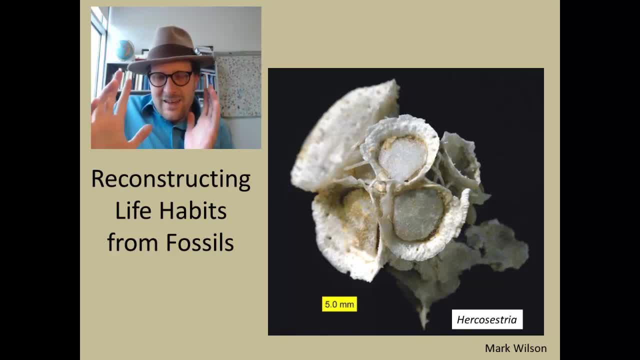 different, but this is totally not like any brachiopod ever you've seen. this is from the permian of texas, um from the guadalupan, and these guys have these, these like little open flaps there, and then they have this like weird strange lower hinge on their um and their bodies and they 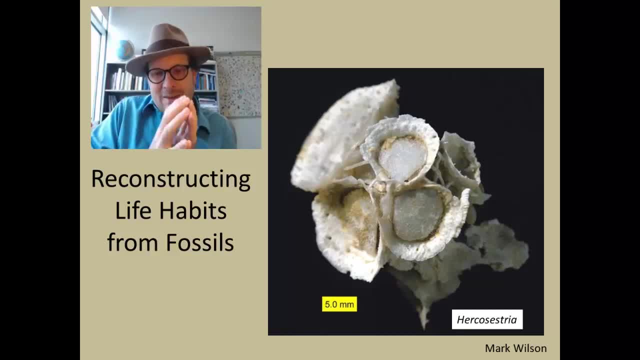 they're all different shapes. you know, brachiopods today tend to be very constrained in terms of their sizes and stuff, and so these guys were brachiopods that decided they wanted to be. sessile corals wanted to be planted firmly down onto the substrate and they form reef complexes during. 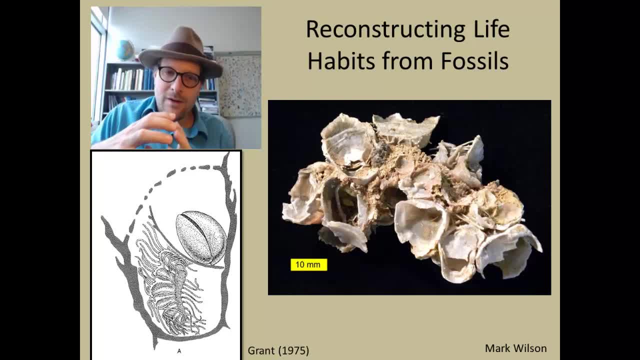 the permian and they're really fascinating. and one of the things that's really interesting is that many paleontologists debated how they actually opened on that hinge, because it's a very weak hinge and we'll talk about brachiopods later on, but they have a very specialized hinge to open. 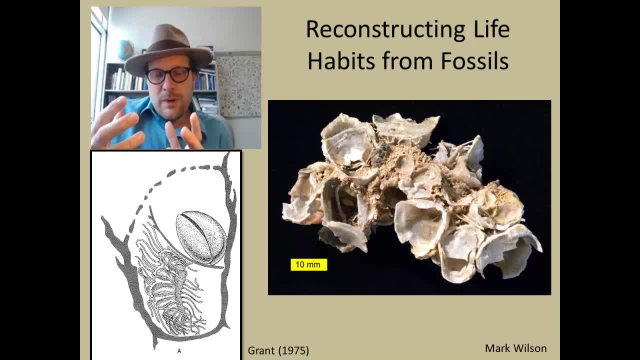 up and close, and so there's this huge debate of whether they opened their hinges or not and how they actually would feed, live in these, in these reef deposits in the permian and there's a fossil that was found, where a brachiopod- another species of brachiopod- got in and was basically living within on top of. 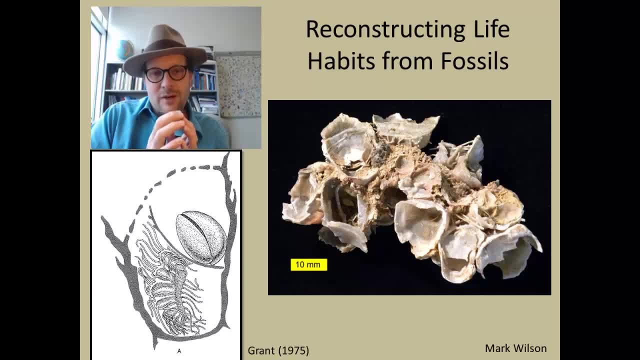 there and they realized something: that this hinge was non-functional. so what these guys would do is they would have their lofaphores, which are the the parts that they bring out to feed, that would sit in there, and they wouldn't open up the hinges, they would just keep it open and that's. 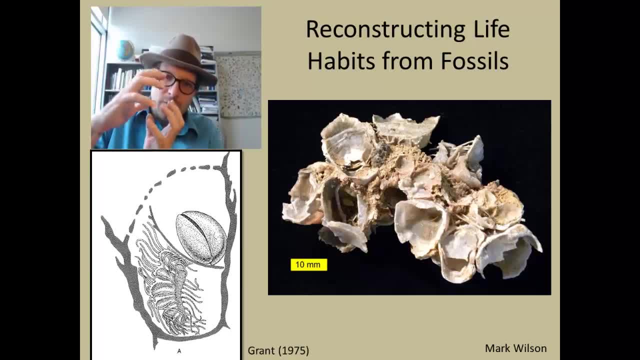 That is how they would feed, but they were using that top end to protect them from predation. They didn't necessarily have to close it or open it, like modern and coeval brachiopods like this one that found itself in this little net that lives there. 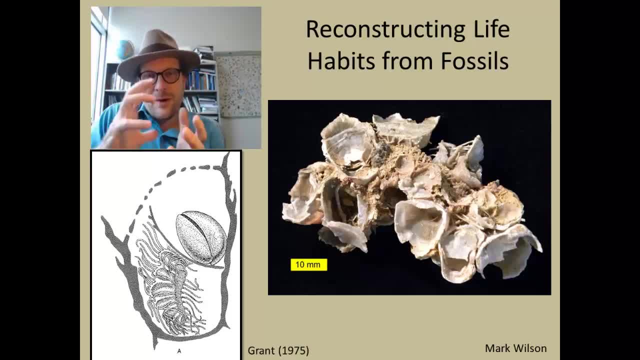 This is a really cool example of an organism that completely changed the habitat and niche that it fit into. They are really cool and fascinating. weird brachiopods- We will be talking about some bivalves that do this as well later on, where they completely 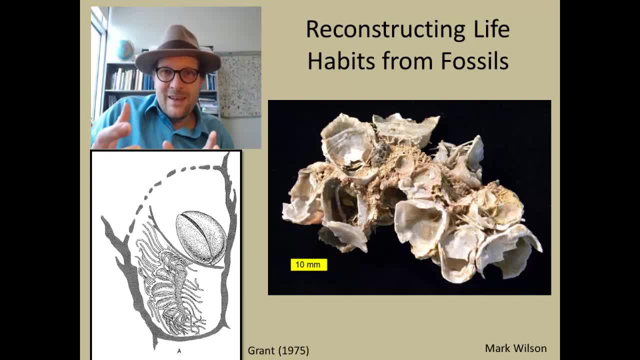 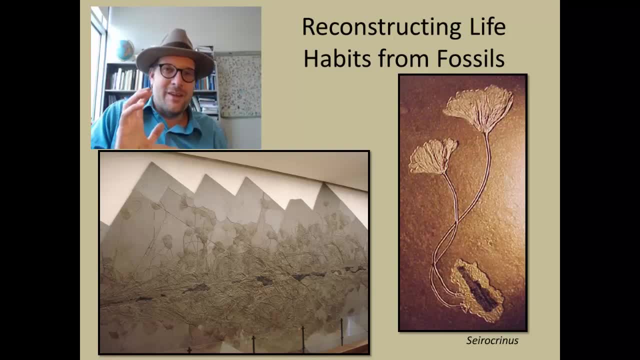 become sessile and more of a coral like creature than the more mobile versions that they had earlier on, or the more normal version, I should say. Another example of a sessile organism becoming planktonic is with this crazy, weird crinoid called serocrinus. 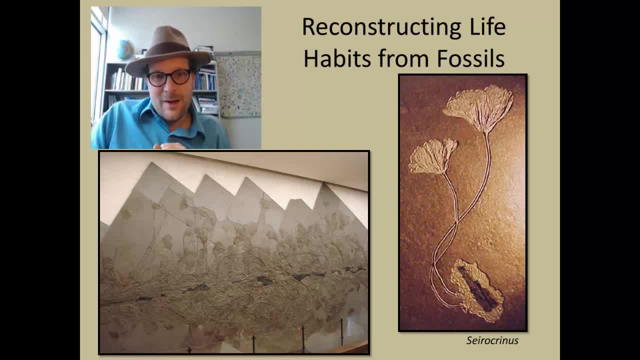 Serocrinus is found in Europe and in the Jurassic. and they are just weird. They are basically like your typical crinoid. These are the sea lilies, and traditionally crinoids are going to be implanted on the sea floor. They are going to have a flowering part that comes up. 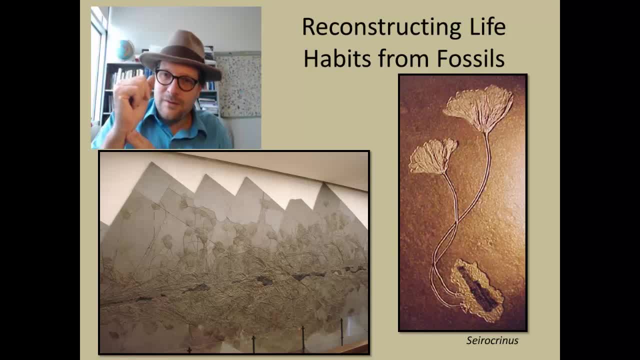 This is the calus that they can feed with their tentacle, like arms. but what these guys did is they hitched a ride on things. They would float, particularly wood fragments, Logs and things would be floating and these guys would attach to them and then dangle. 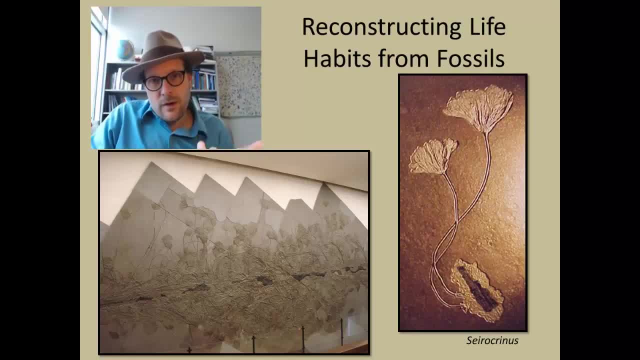 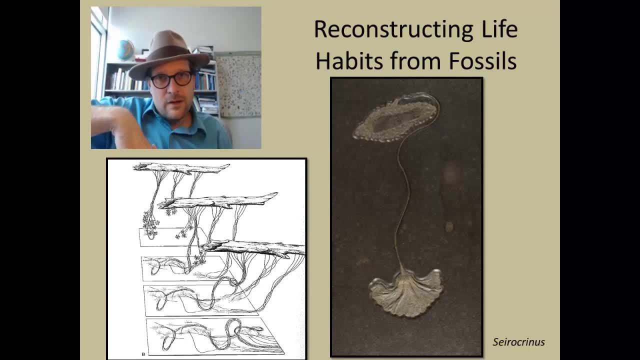 below the floating logs or organic material that would float. They would drift along the ocean, dangling upside down and feeding in the water column. This is a way of a sessile organism becoming mobile and being able to move around the landscape. There are some other wonderful examples. 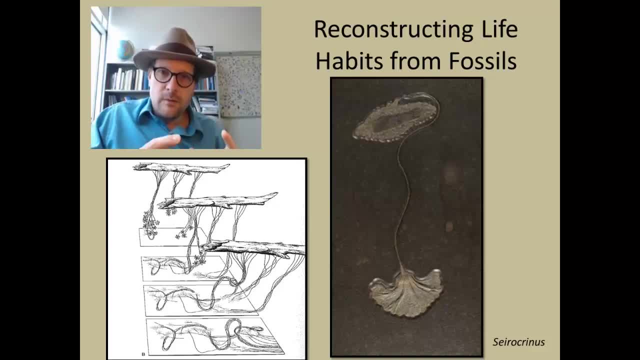 We will be talking about sessile organisms that became more mobile as they evolved through time. Another example of how strange and weird some of these habitats can be: Some organisms like crinoids, that typically are going to be sessile and tied down to the 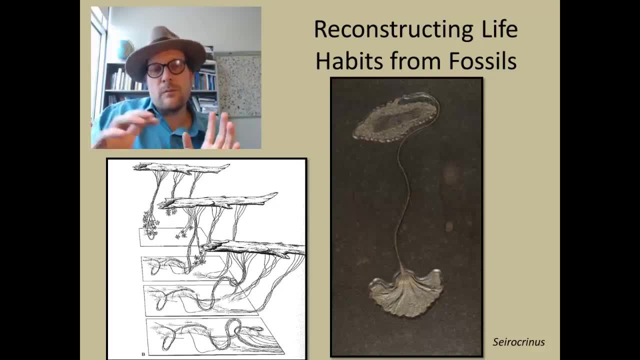 ocean floor can suddenly find a way in which they can become more mobile and move around within the ecosystem and change their niche and change their habitat to do something new and unique. One of the things you also want to look for is not necessarily just fossils, but also trace. 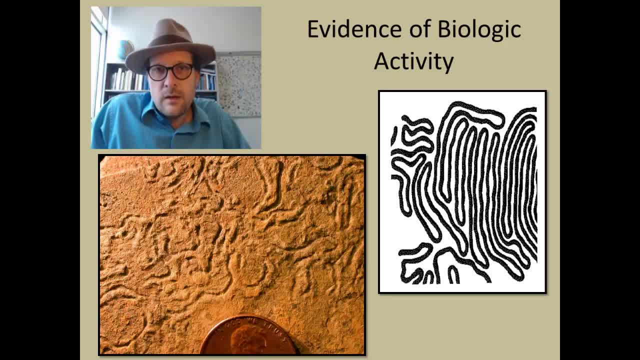 fossils or evidence of biological activity that is going to be very key to understand and reconstructing ancient marine environments. Trace fossils- we will be spending more time on trace fossils later on this semester- are really important. These are marks that are left behind of grazing, of snail grazing. 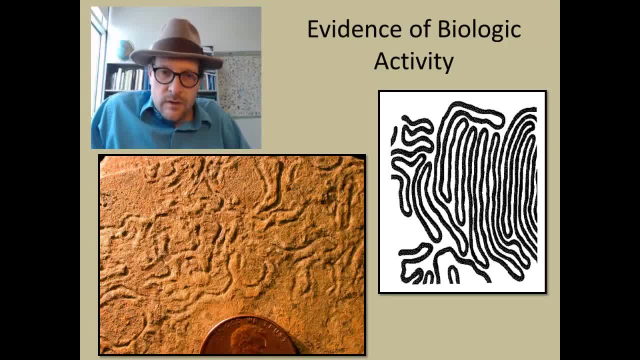 These are gastropod marks or grooves that existed on this muddy beach, where these snails went across and were feeding and grazing. as they moved across the landscape, They left behind these grazing traces. You may not necessarily capture these gastropods, Maybe these particular gastropods don't have shales or hard parts, but you get the indication. 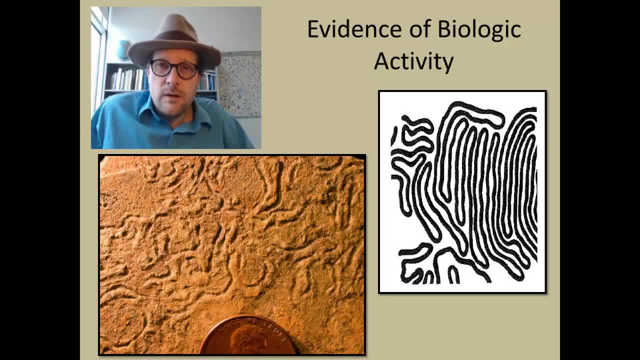 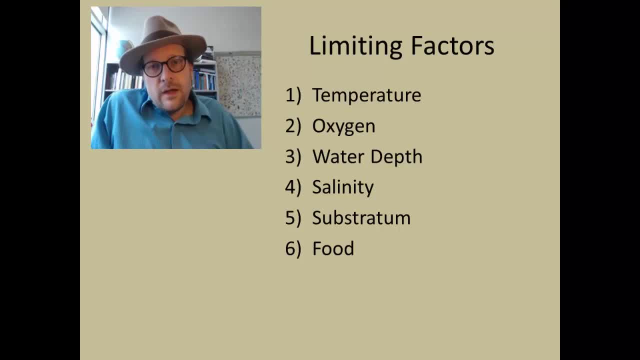 that they are there from the trace fossils. Trace fossils are very important to bring forth whenever you are doing paleoecological studies. Now I am going to talk a little bit about limiting factors. These are some of the things that we can use. 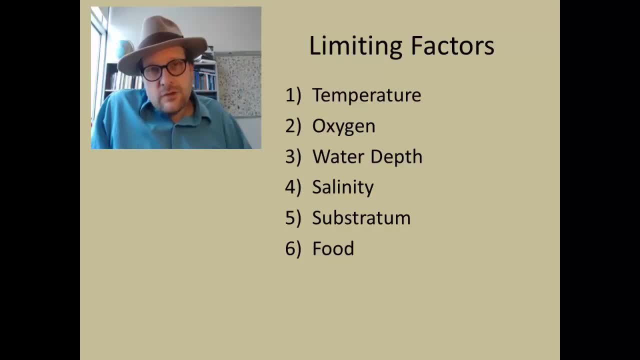 Now the fossil record to try to get at in ancient environments, things like temperature or climate, the amount of oxygen in the water, the water depth, the salinity of the ocean, the substratum, and also something about the food or the food pyramid, food availability. 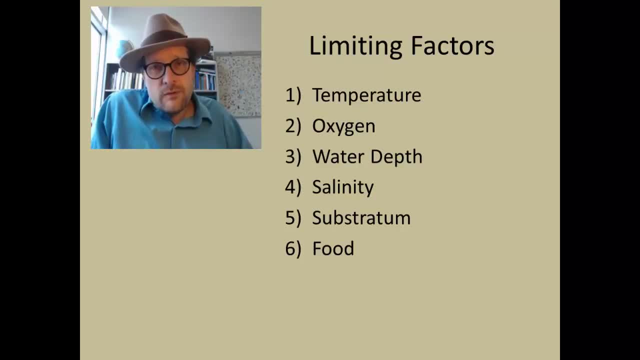 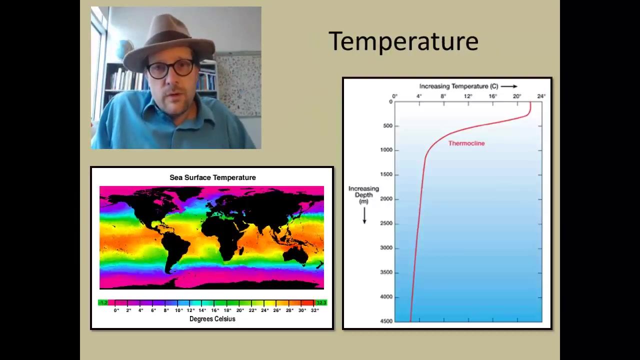 or nutrition that might be available to the organisms living at that time. So when we are reconstructing The environment, These are things that we can actually use- the fossil record to use to reconstruct what the ancient marine system was like. So let's look at these real quickly and run through them. 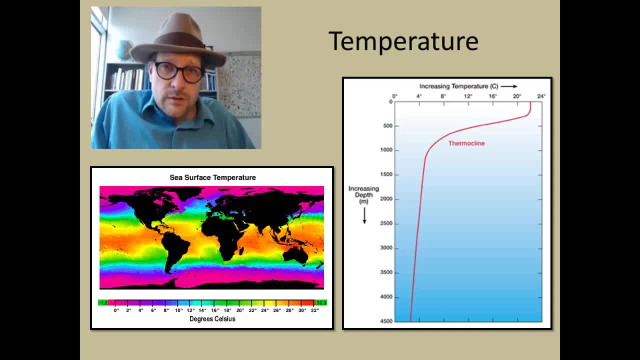 So temperature varies quite a bit in the world's oceans. Sea surface temperatures are the warmest around the equator, And as you move towards the poles the sea surface temperatures drop off and become more cold. But the other thing to remember is that as you go deeper in the ocean, temperatures are 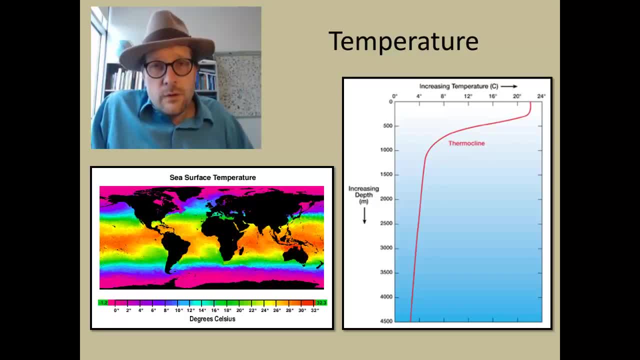 also drop and become colder. So the coldest ocean waters are found near the poles and at the deepest part, the abyssal plains, the very abyssal, deepest parts of the ocean, And those are going to be the coldest And this is going to be important when we are reconstructing climate through. time is 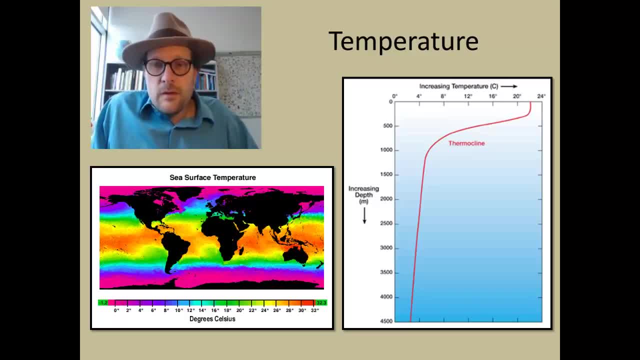 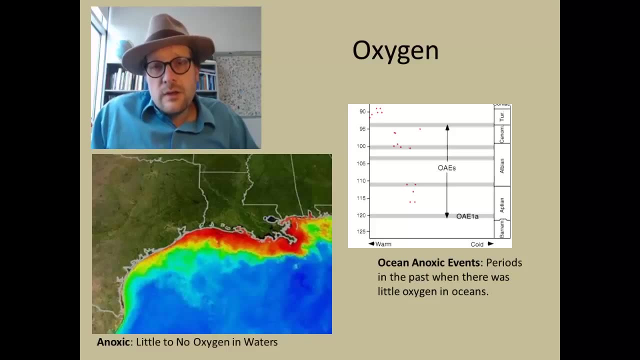 knowing where you are in the water column. This pattern of warm surface water going down to cold water is called the thermocline when we look at it in the water. Another thing that is really important is oxygen. Oxygen is needed for many animals that live in the ocean, whereas many of the photosynthesizing 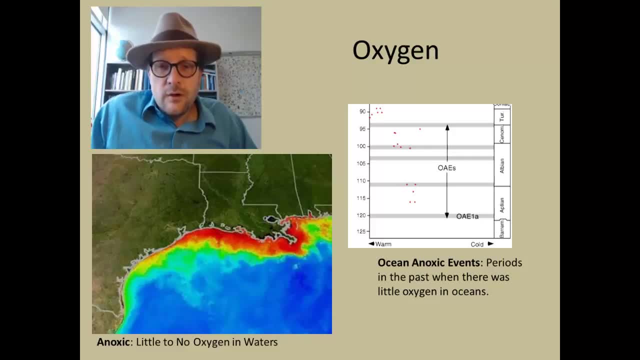 organisms don't require oxygen. Oxygen can be depleted, and when oxygen is depleted in the ocean, we refer to these as anoxic conditions. Anoxic conditions happen in many parts of the ocean today. A lot of times they happen, For example, along the coast of Louisiana, along the Mississippi Delta. this is caused 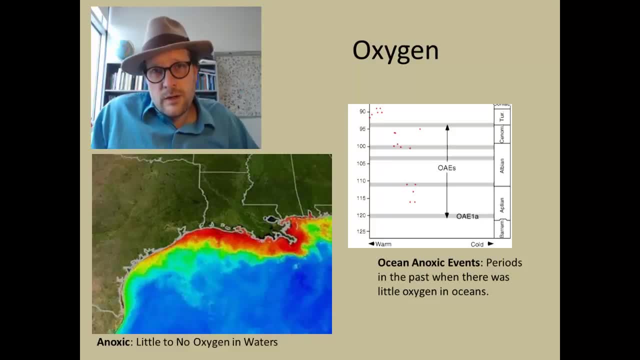 by organisms, photosynthesizing organisms that bloom like a lot of the algaes and they become extremely common and then they die and they sink down And organisms start to feed scavenging organisms on those algae blooms and they use up all. 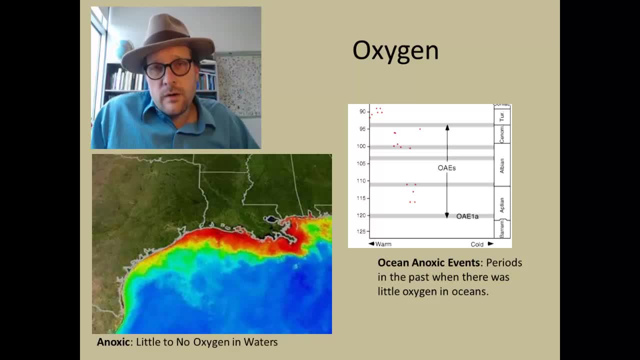 the oxygen. So there is no more oxygen for many organisms, Organisms like fish, crustaceans- and this is a big issue with many fisheries and shrimp farms and stuff along Louisiana is, when you have these anoxic conditions, it means that 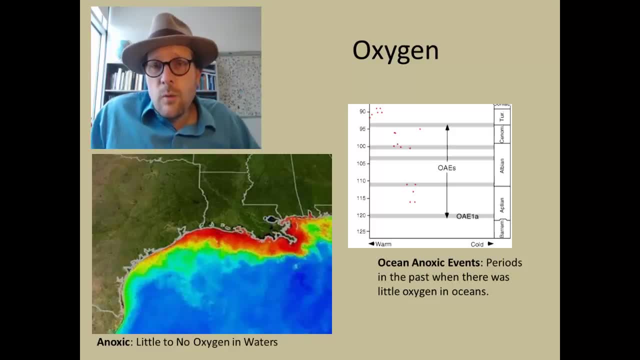 all those organisms die. They just don't have enough oxygen in the water to live. Anoxic periods have happened in the Earth's path. There is a whole bunch of anoxic water during the Cretaceous periods and these are periods where you get a lot of organisms dying out and they are also characterized by changes. 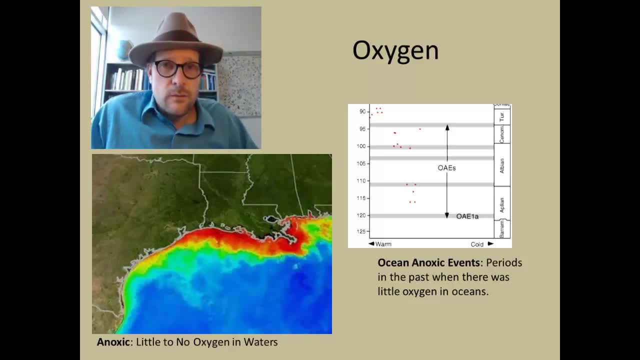 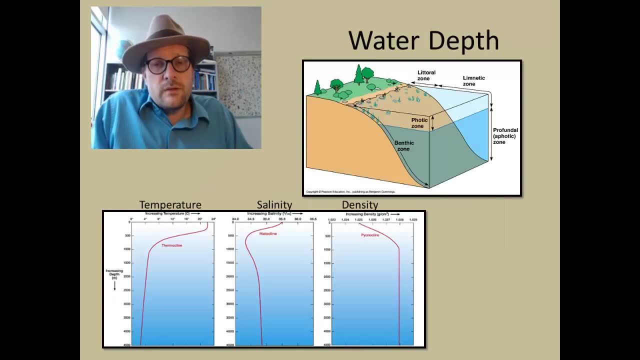 in the water chemistry as well. So anoxic events are something to be aware of because they can have a pretty profound effect on the ecosystems. Water depth is one of the ones that I think paleontology has the best way of getting at water depth, and that's because organisms are really dependent on how deep they are. 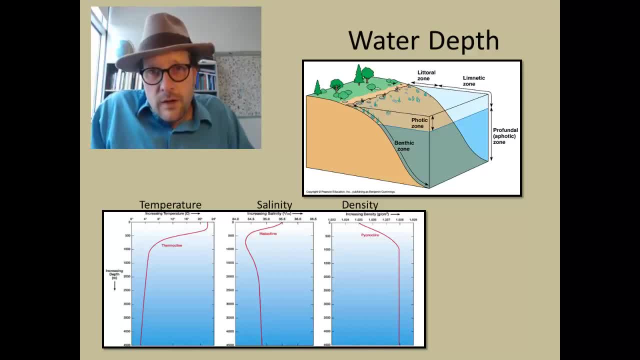 So the photoxone is really important, because the photoxone is how far light will travel down. So many organisms have to live within the photoxone. They need that light to live and exist. So as you go deeper in the ocean, if you're an organism you have to change the way in. 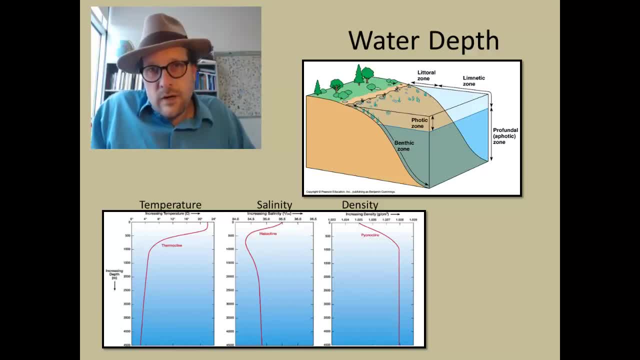 which you make your living, and you have to figure out a way to live in the dark. basically, if you're going to be down in the benthic zone of the aphotic zone. so the deeper, darker waters. The other thing about water depth is that as you go down, 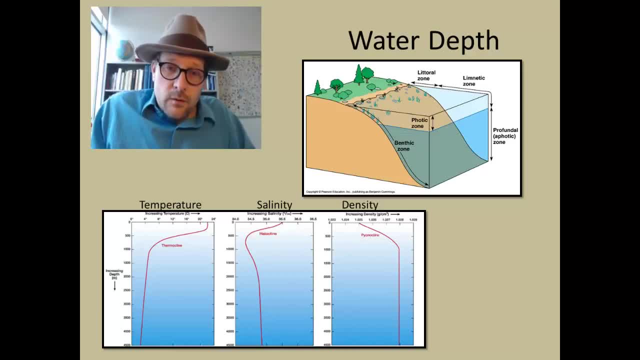 Temperature changes, You have to worry about salinity. So the saltier waters are near the surface, so there's greater evaporation and deeper waters tend to be a little bit more fresh. but there's what's called a halocline in determining. 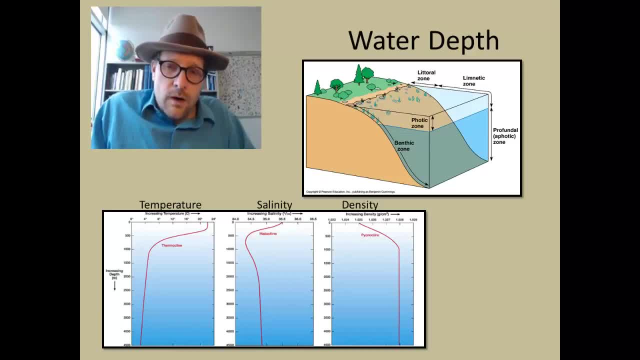 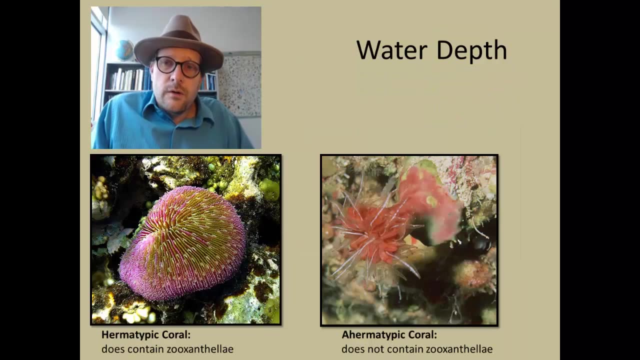 salinity And also density. So the water near the surface is less dense than the water at deeper depths and that has to relate to the changes in salinity and the changes in temperature that reflect the differences in density. Now we'll be talking about corals and the importance of water depth to corals, but there 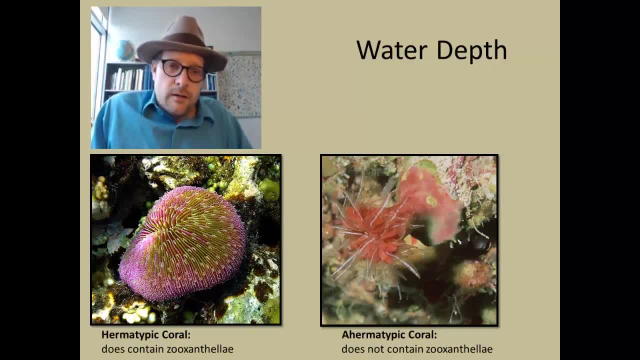 are many corals that rely on a symbiotic relationship with photosynthesizing bacteria. These corals are called the hermotypic corals. Hermotypic corals are the ones that contain this thing, called these bacteria, called zonanthia. 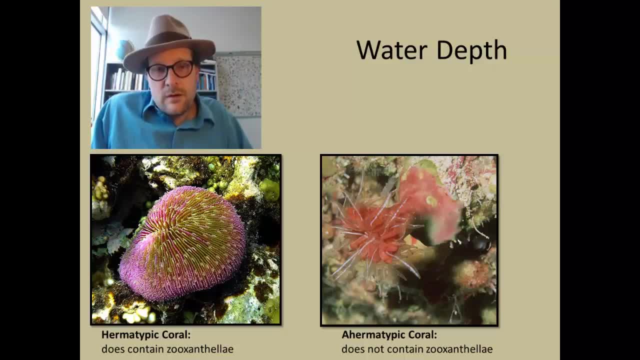 Zonanthia are photosynthesizing bacteria that live within the coral and they need to be in the photic zone for that bacteria. So the coral itself feeds on these bacteria and the bacteria basically gets its energy from the sun in the photic zone. 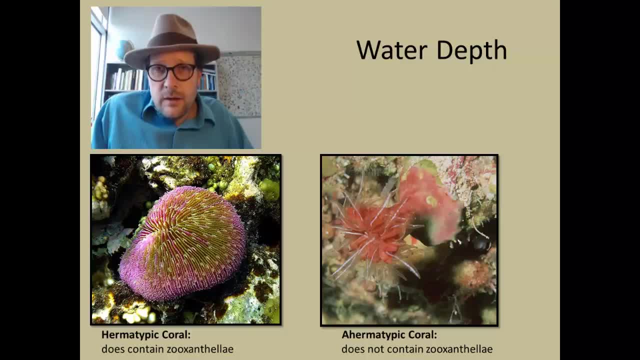 So if you ever hear of coral bleaching- I'll talk about that later on- that's when the coral loses its zonanthia and then it basically dies of starvation, because there's no none of this photosynthesizing bacteria to feed on, and so that causes the corals to die. 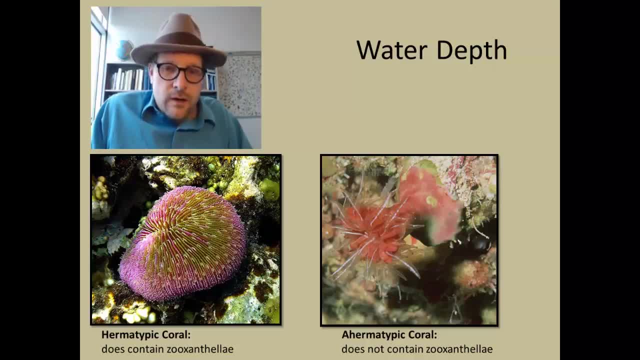 A hermotypic corals. Hermotypic corals are corals that do not contain zonanthia and these are at deeper depths. So these are corals that live at very deep depths and they don't have the bacteria that. 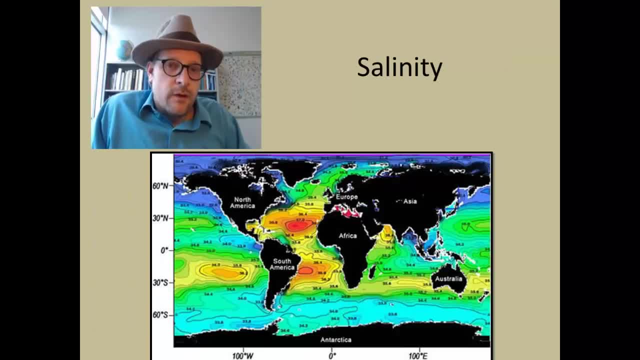 require photosynthesis. Salinity varies quite a bit across the oceans. There's different parts of the ocean where salinity is very high, and there's certain parts of the ocean where salinity is very low. Salinity tends to be highest where there's the greatest amount of evaporation. 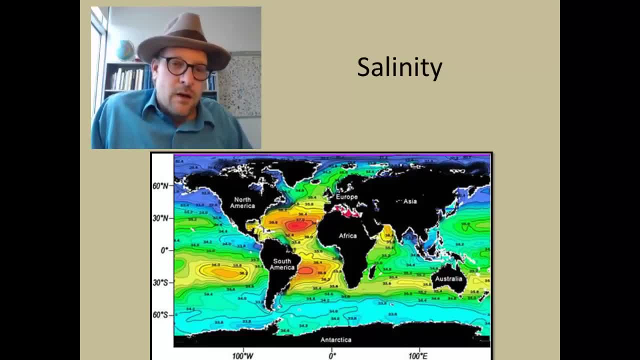 This includes, like the Red Sea, the Mediterranean- Okay- As well as some of these open parts of the Atlantic Ocean in the middle of the ocean, gyra. So these are areas in which there is significant evaporation going on. Places where the ocean water tends to be more fresh is in Southeast Asia, where you get a. 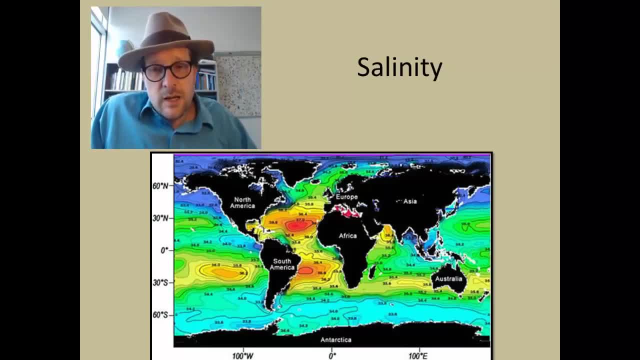 lot of runoff of fresh water from these monsoonal conditions. that can happen across India and Southeast Asia, as well as in polar areas where you have a lot of glacial snow melt and sea ice melt, But it brings in lots of fresh water seasonally into the oceans. 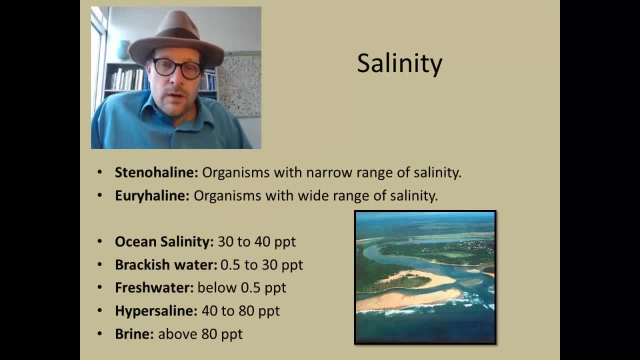 So salinity is a major factor. Now, organisms can either have a great tolerance in salinity or they can have a very narrow tolerance in salinity. So steno-haline organisms have a very narrow range of salinity, whereas urihaline organisms. 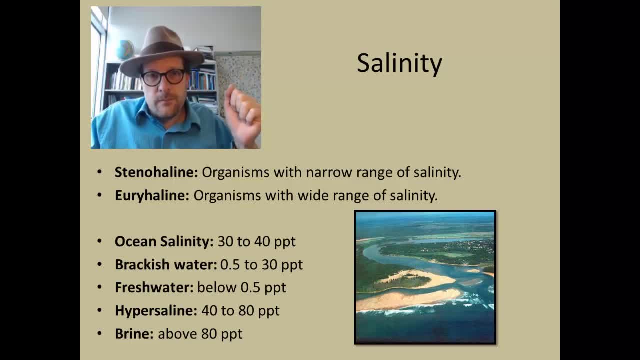 are organisms that can live in a very wide range of salinity. So to give you some salinity numbers, So ocean salinity is between about 30 to 40 parts per thousand. Brackish water is about 0.5 to 30 parts per thousand. 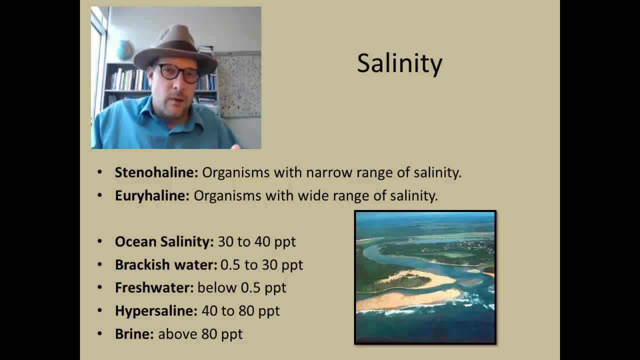 So brackish water is going to be where you're going to find fresh water coming out into the ocean. So these are estuary type environments. Fresh water is where salinity is below 0.5 parts per trillion, parts per thousand. 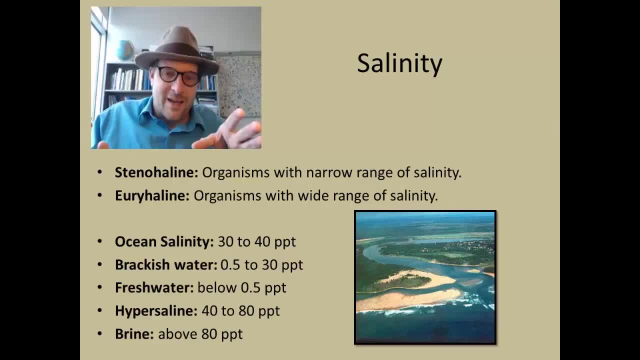 And then hypersaline are where you get like 40 to 80 parts per thousand, So very salty places. This is hypersaline. you get like in the Great Salt Lake here in the United States. And then you get brine. Brine is above 80 parts per thousand. 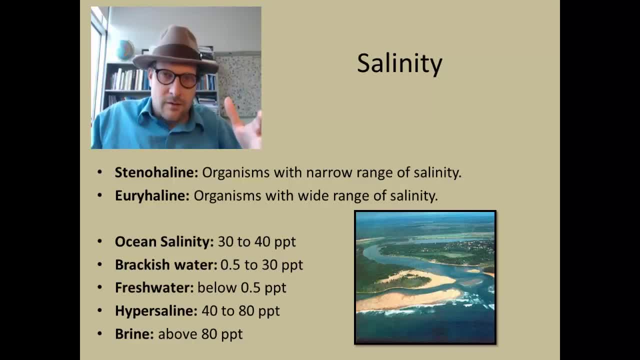 So these are very salty places, like the Great Dead Sea in Israel, Some places like that where it's very salty. Now, many organisms can live in certain salinity levels, but brine conditions are probably the most severe. Only just a handful of organisms can live in brine water. 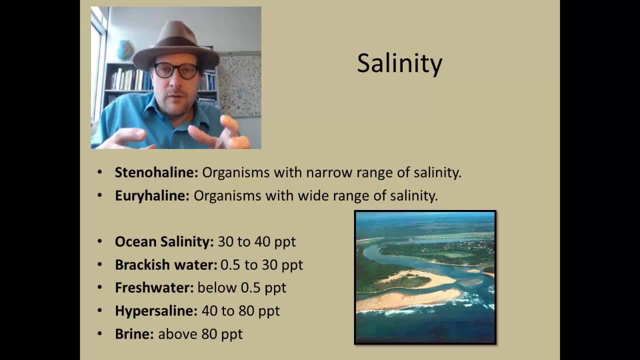 So salinity is very important in terms of where organisms can live, And so knowing those tolerances and the limiting factors in the fossil record will help you reconstruct the salinity in the ocean- Another really important one that we usually don't consider but is very important for the 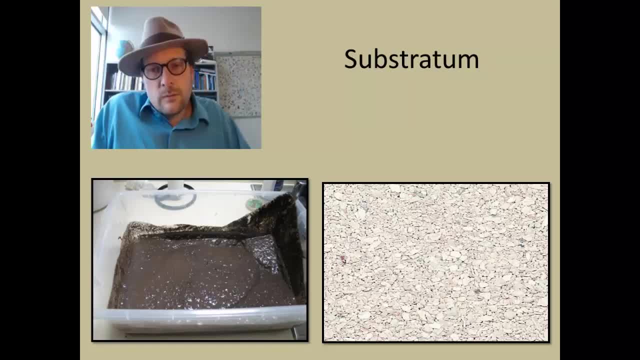 organisms that are living in the marine ecosystems is the substratum, That is the surface that they are living within. So you can imagine mud, Mud, Mud substratum. Living in mud is going to be very different than living in sand or gravel. 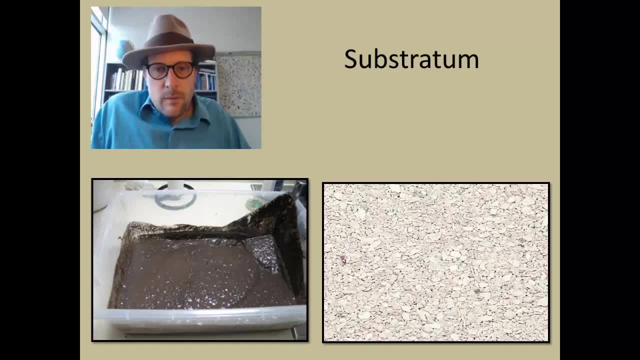 So if you're along a gravel beach or sand beach, it's going to be a very different environment than if you're living in a muddy sort of tidal flat, And so organisms tend to live in different environments based on the substratum. So many mollusks will like burrow down. 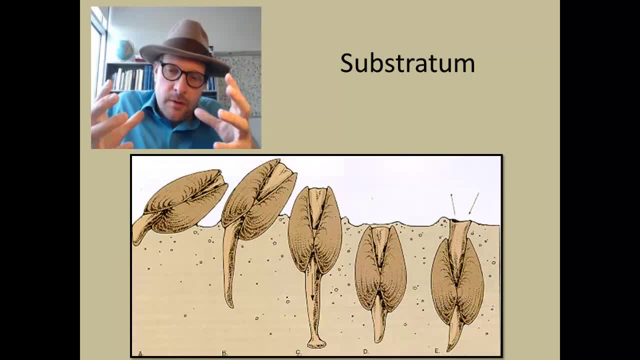 We'll talk more about this when we talk about them in more depth. but they'll burrow down the substratum. They need to live in muddy areas and they need a certain amount of. if it's too muddy or too mooky, then they may have trouble living in that type of habitat. 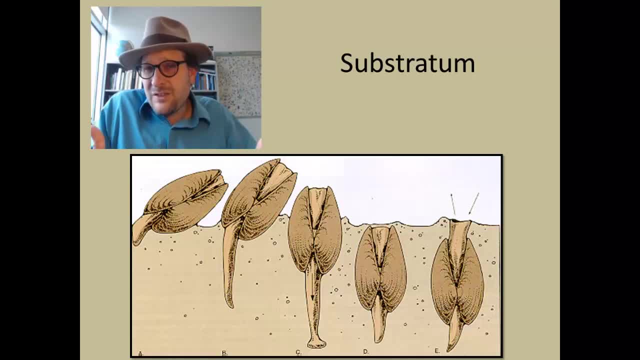 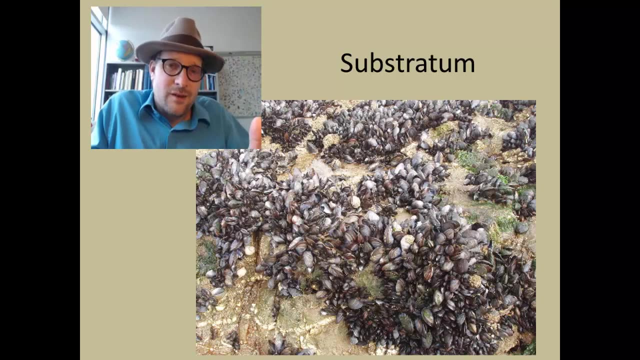 Whereas if it's more sandy they might find it more beneficial. So imagine sand dollars needing that sand, and so the substratum is pretty important for their feeding and the way that they make their living, their niche. Some organisms, like mussels of course, can burrow into hard rocks and stuff and they 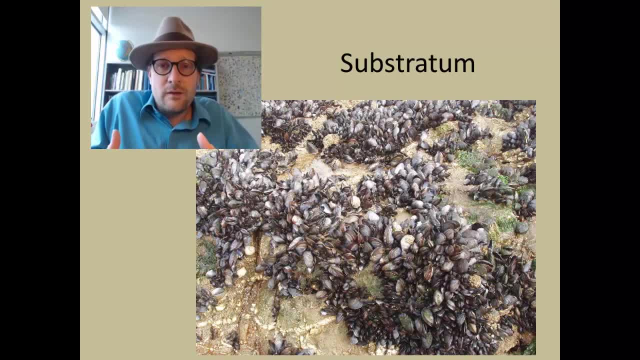 don't necessarily need mud. They actually need, like, a rocky surface where they can attach to and grow from, And so that becomes their substratum. So we'll talk more about substratum when we talk about these very smallest groups and the way that they attach to the substrate. 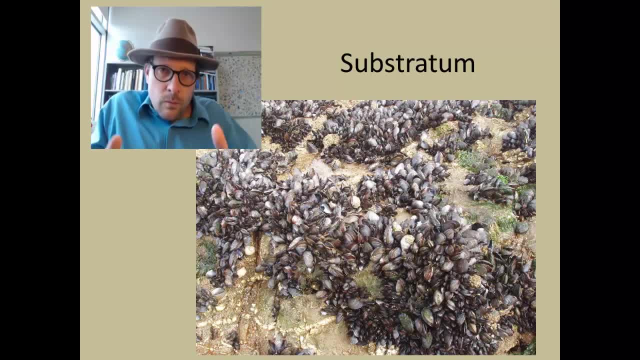 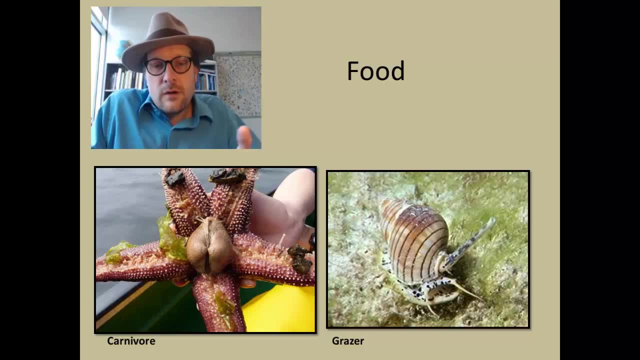 But these are very important things to consider when you're reconstructing this ancient marine environment. So food is another limiting factor that we should consider. So understanding each of the fossil organisms' role within food And how they actually get their food is going to give you a greater insight into reconstructing. 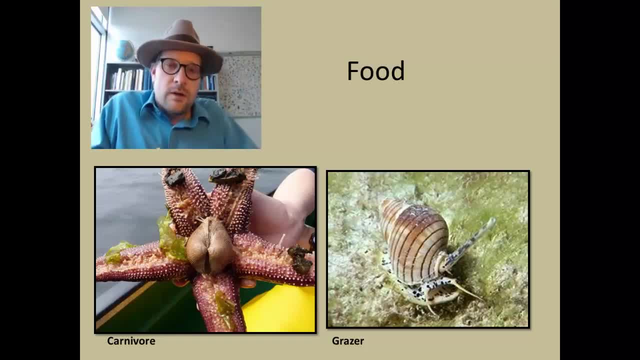 this ancient marine environment. So you can have organisms like starfish that are carnivores and that way they're going to be feeding on other organisms. Or you can have organisms like this gastropod, this little snail that's a grazer. 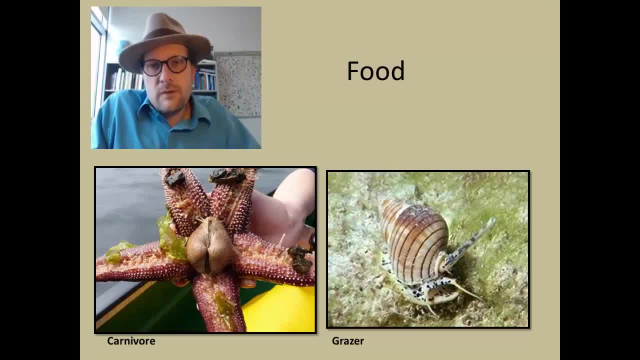 And so these are very different organisms and you might find them in very different environments, And so finding them is going to give you a greater insight of what the ancient marine environment was like. So hopefully this video kind of enables you to think about some of the things that paleontology. 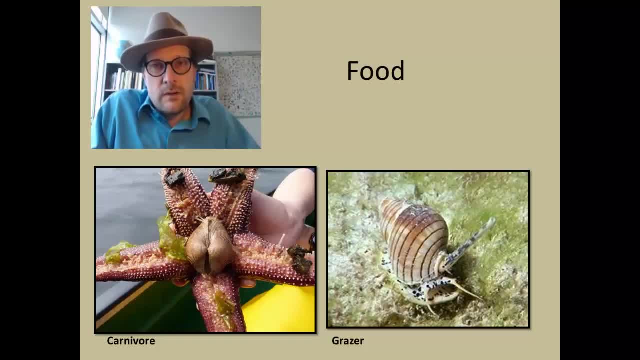 can bring forth when you're reconstructing the ancient marine environment. All right, next time in lecture 10, we're going to talk a little bit more about cyclic perturbations that can happen in the marine system and how communities can recover and change and how 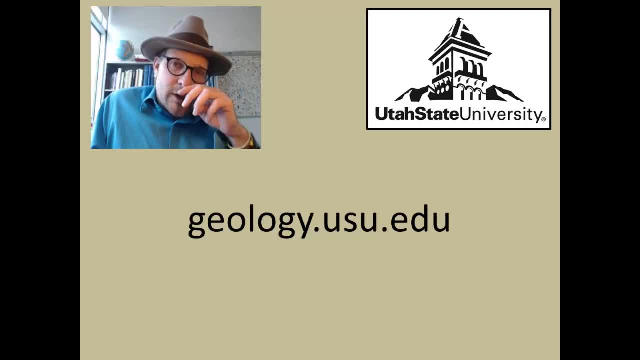 we might be able to see that in the fossil record. So thanks for watching. If you're interested in taking a course in geology at Utah State University, you should check out the department website at geologyusuedu, And if you're interested in who I am and my own research, you should check out my website. at benjaminbergerorg.